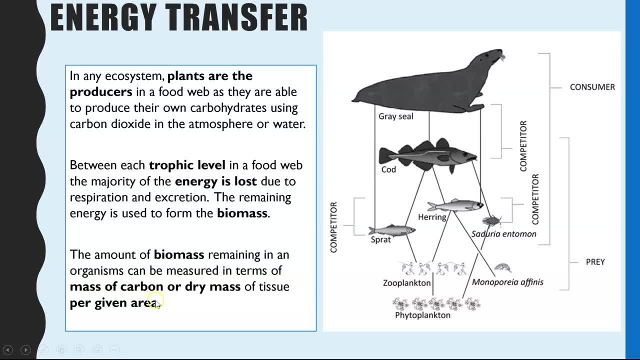 be measured in terms of the mass of carbon or the dry mass of tissue per given area. so sometimes you might get questions where they tell you how could you work out the biomass of a plant? so you'd need to remove all of the water to make sure it was just the dry mass, and in that way you know you've. 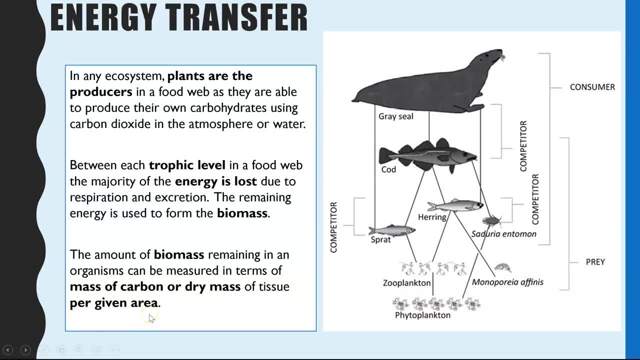 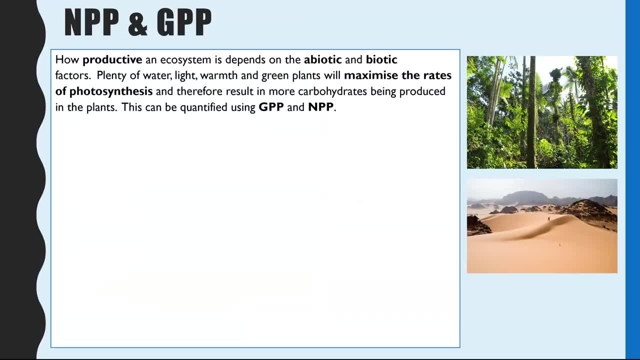 got the mass of the carbon and we do it per given area, just so it's a fair comparison between different sized organisms. so NPP and GPP- these will be two new terms compared from GCSE, and this is linking to how you can quantify how productive an ecosystem. 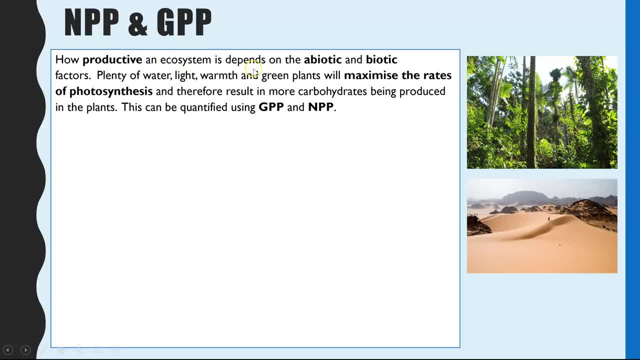 is, and the productivity of an ecosystem depends on how favorable the abiotic factors and biotic factors are. so if there's plenty of water, there's a high light intensity and it's nice and warm, there's lots of green plants available. all of these abiotic and then the green plants, biotic. 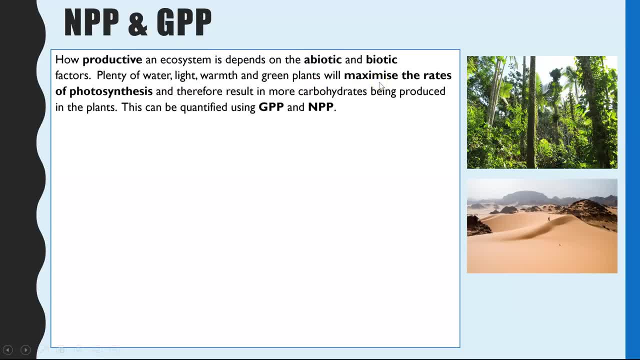 factors will help to increase the rates of photosynthesis, and photosynthesis is how we're going to track this, and the reason why I ask that we look at them straight up is because we just don't get a clear picture of what you just see in a graph that's either a77 or an F2A5, so that's your biasOnse of the food chain. 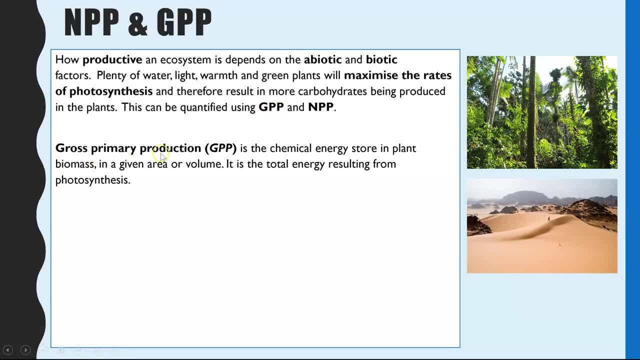 GPP is gross primary productivity or production, and this is the chemical energy store in plant biomass and it's given per area or per volume. so again, it is a fair comparison between different ecosystems. So what we actually mean by this is it's the total energy resulting. 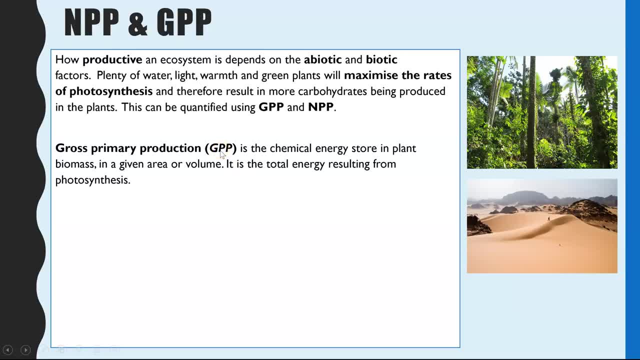 from photosynthesis. So GPP is the total energy entering your food chain as a result of photosynthesis. Now, in comparison, NPP is the GPP, but it takes into account the energy lost in respiration. So it's the total amount of energy from photosynthesis minus the energy that will. 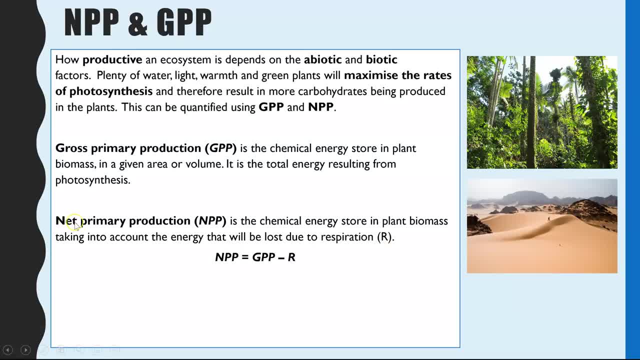 be lost in respiration. So what that means is the net primary productivity or production, that is, the chemical energy that will therefore be left over to create new biomass in the plant. So that is really what we're interested in: how much NPP is there? because that is the amount of energy that can then be used. 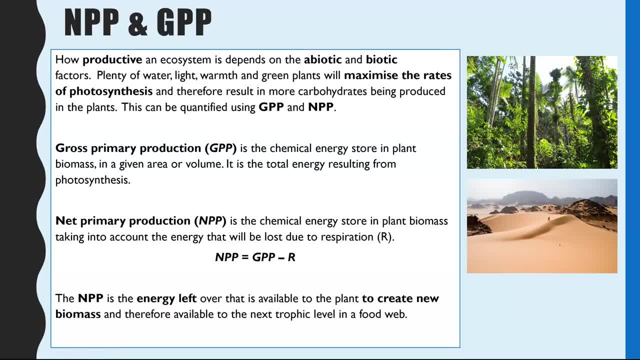 to create biomass, and the biomass is what can be passed on to the next trophic level in a food web. So I've got two examples Here. we've got the rainforest, we've got a desert ecosystem and the top one, the rainforest. 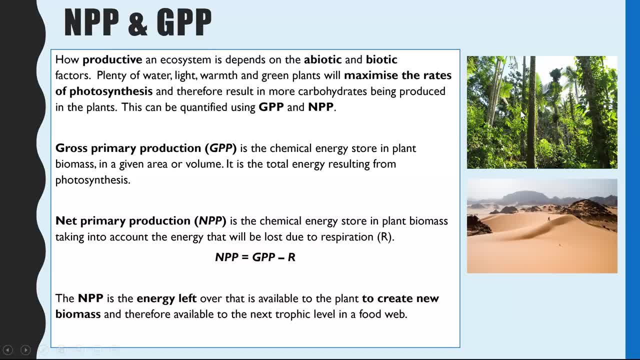 because we have plenty of water, lots of green plants. they both have lots of light availability, but the top one will have far more photosynthesis So it will have a much, much higher GPP. It will therefore have a higher NPP, So a rainforest ecosystem will be far more productive compared to 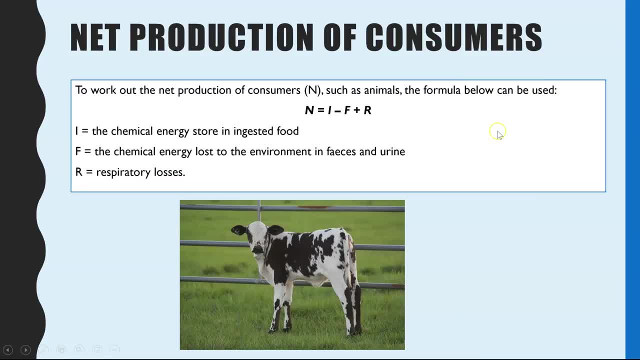 a desert. So another calculation that you could be asked to use is one to work out the net production of consumers, this time instead of plants, And it might seem quite straightforward formula, but they've thrown it onto the new spec now. So if you were to use it, or even state it in an exam question, it 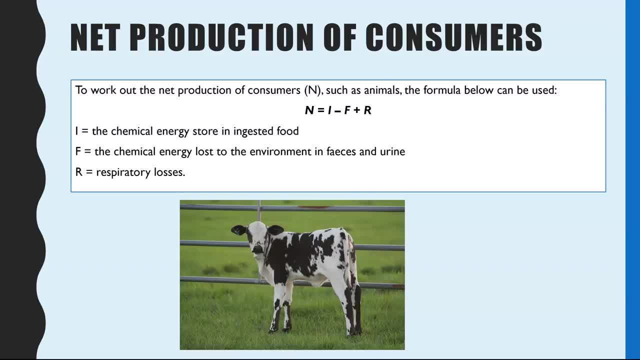 could be worth a mark. So what this is looking at is taking into account the amount of energy entering and exiting the consumer and therefore looking at how much energy is left over that can be converted into new biomass or new cells in the animal. So the I part of the formula is the energy ingested in. 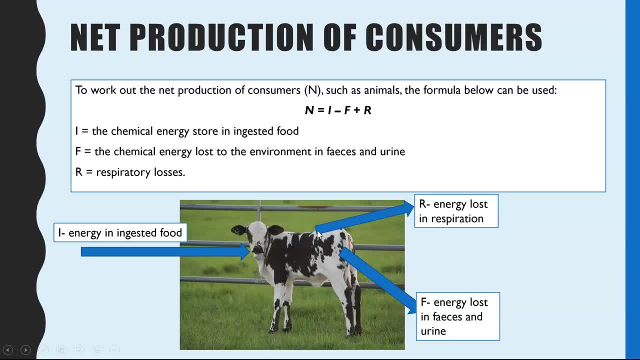 food, So it'll be our chemical energy from food. You then have to look at how much energy is lost in respiration and how much energy is lost in faeces and urine, And this wasn't in the previous formula- because plants- because plants do not produce feces and urine, so that's why there's an extra component to this. 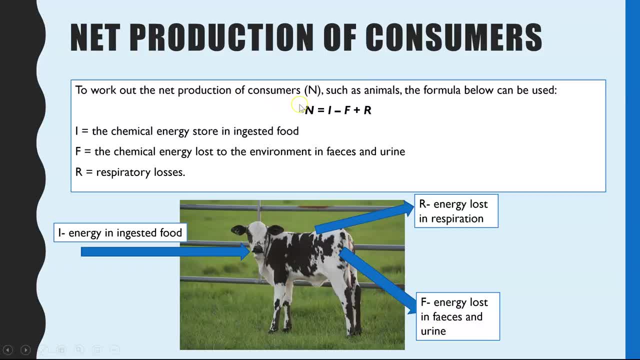 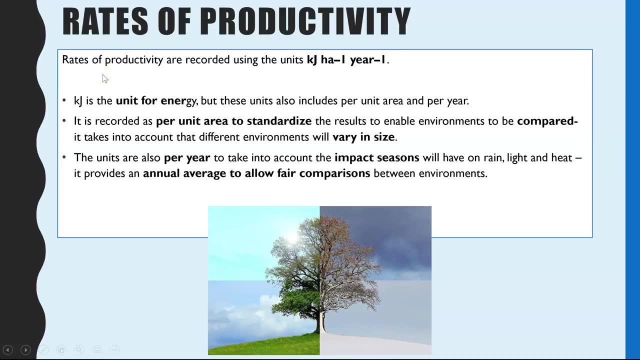 formula. so n, which is the net production of consumers, is whatever you have left when you look at what goes in minus what comes out. so the last thing is these rates of productivity. if you were going to compare how productive two different ecosystems are, there's actually three components to the units you would use in your calculation and quite often you could be. 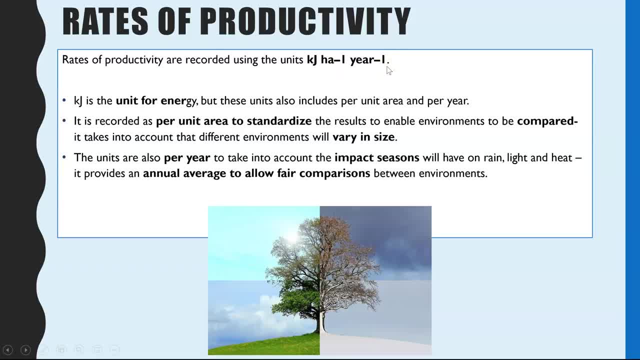 asked for two marks to state appropriate units or you could be asked to justify all the components of the units. so this is actually quite important for this topic. so we have kilojoules now. i've used here per hectare but that could be per meter squared and we've got per year. 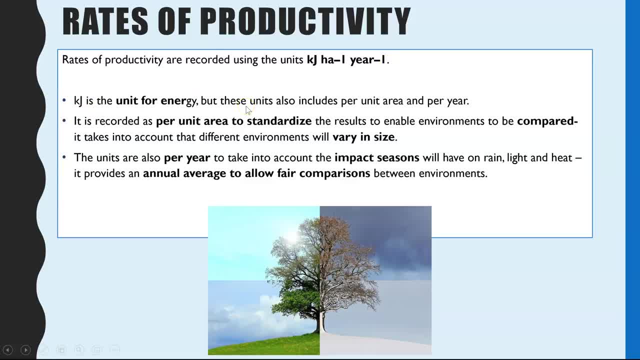 so kilojoules is the unit for energy, so rates of productivity. we said we're looking at how much energy is entering the food chain. so that's why kilojoules is in the units, because it's a unit for energy. but we've also got per hectare there and that is an area, so we have to do per unit of. 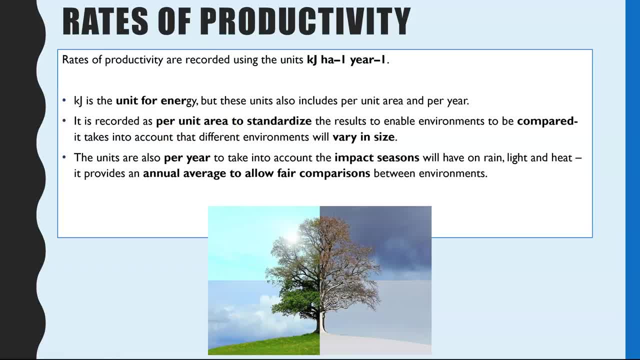 area that you are studying, and this is to standardize your results, because it's not going to be a fair comparison if you're looking at the rate of productivity in a very small field compared to an entire rainforest. so we have to do this, divided by 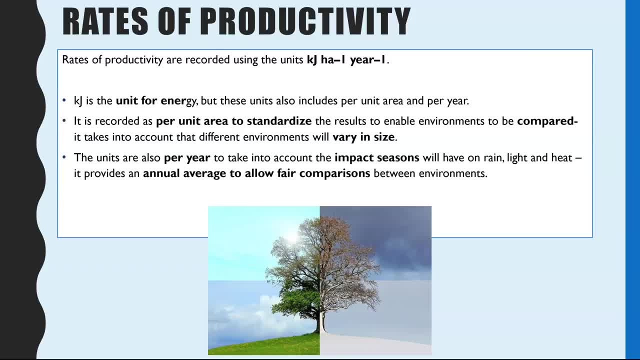 the area that you're studying or per unit area. so it's standardizing the results and therefore we have a fair comparison. similar idea here why we do it per year, and that is again so it's a fair comparison, but this time it's taking into account the fact that throughout the year,